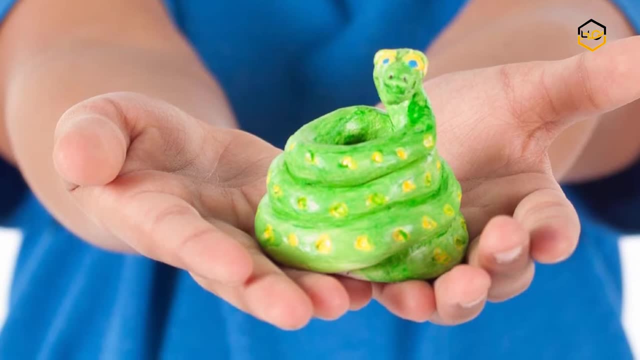 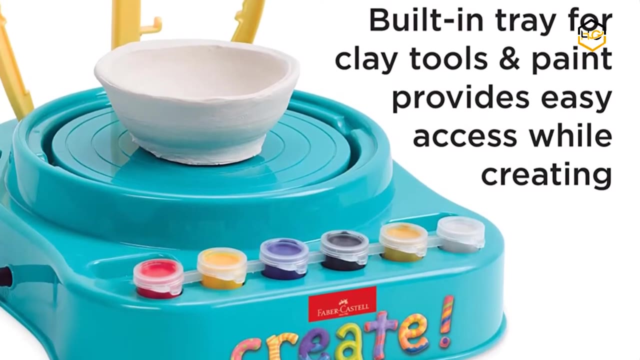 unique gift for kids that will teach and inspire. The Faber Castell Pottery Wheel provides steady and sturdy power that will hold and spin, with enough clay and pressure to create mugs, pots and variety of knickknacks. The premium quality clay included in this kit comes from nature, rather 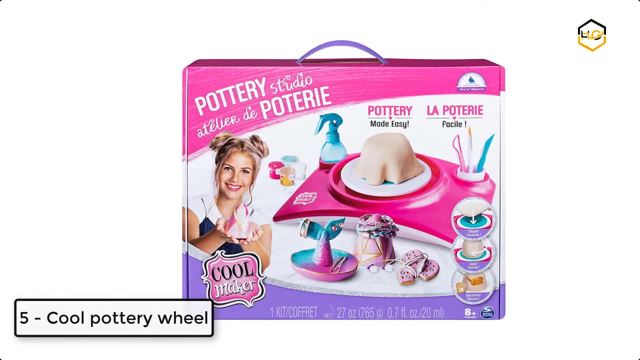 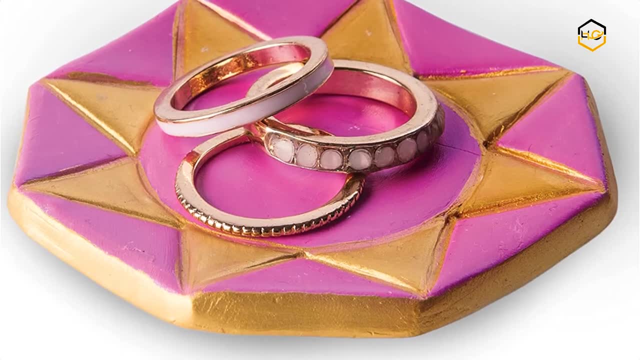 than being manufactured. At number 5 we have Cool Pottery Wheel. This innovative kids pottery wheel studio makes crafting and designing clay projects incredibly easy and fun for kids to do. The cool maker has turned pottery upside down. simply place a clay disk onto the turntable. gently spray it with. 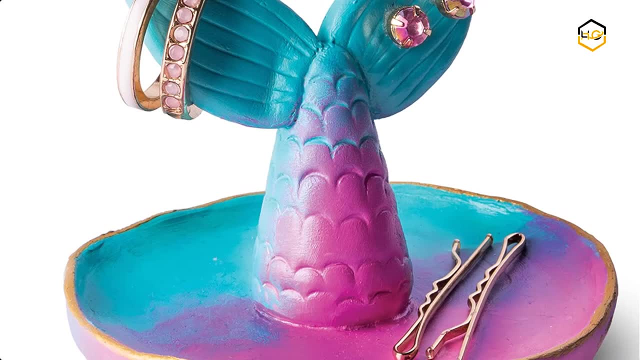 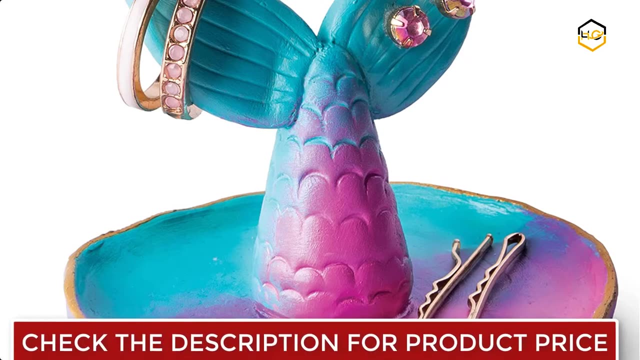 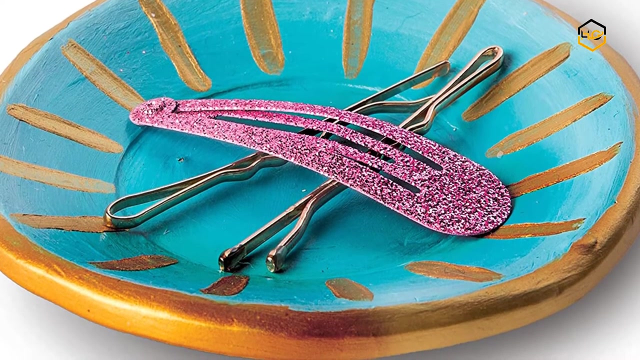 water and watch it spin and take shape in your hands. Coolmaker Pottery Studio's unique design helps you create perfectly shaped pottery by letting gravity do the work for you, And once air dried, the creativity really begins. This pottery kit for kids comes with multiple sculpting tools and 5 brightly colored metallic paints. so you can 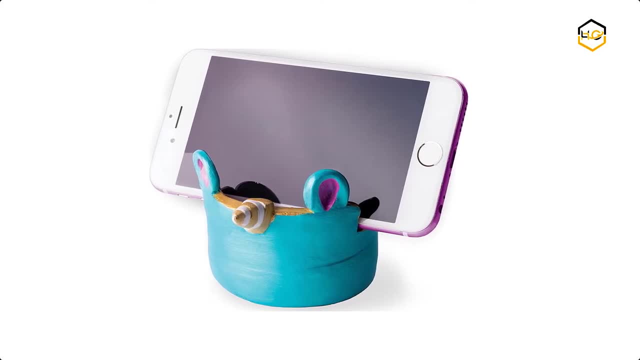 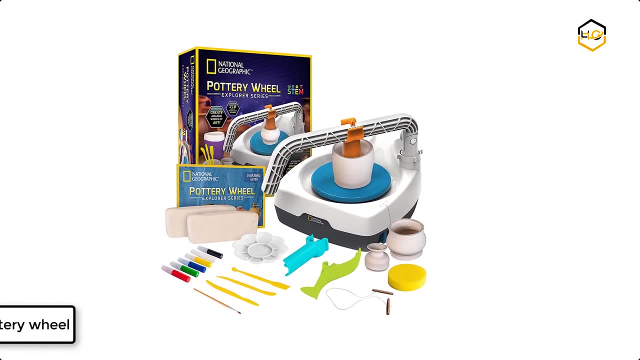 quickly customize each creation for a truly unique look. It's pottery made easy. The Coolmaker Pottery Studio comes with everything you need to start right away. At number 4 we have National Pottery Wheel. You can create your own decorative air dry pottery with 2 pounds of air dry clay, 3 arm. 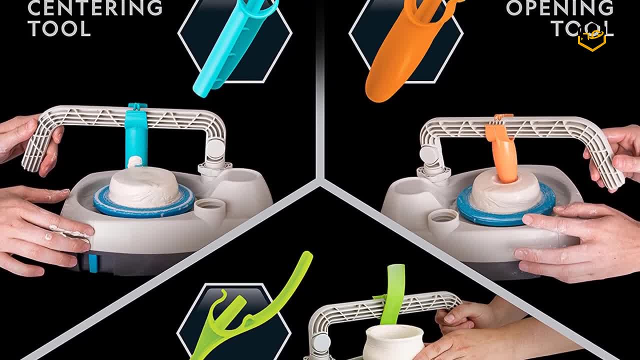 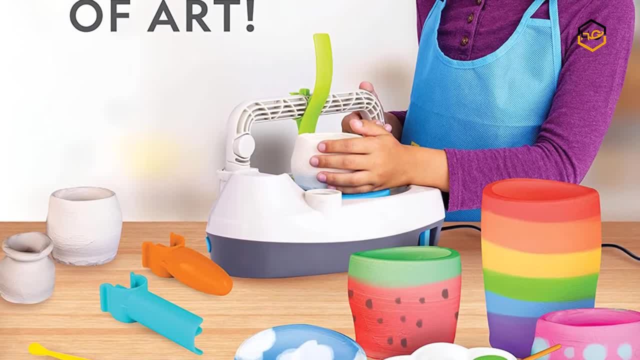 attachments: 3 sculpting tools, 6 paint colors, palette, brush, apron and much more included. This pottery wheel is specially designed for beginner potters of all ages, with innovative arm tools to assist in centering, opening and shaping your clay. The pottery wheel for beginners. 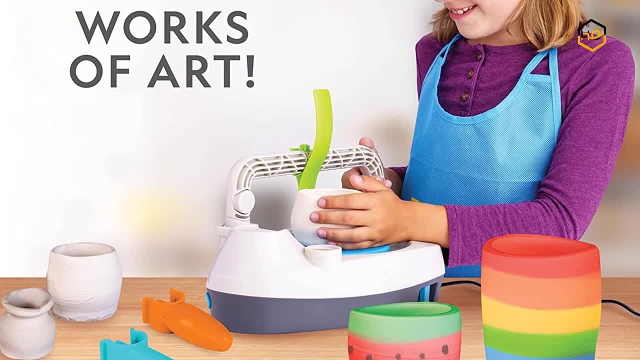 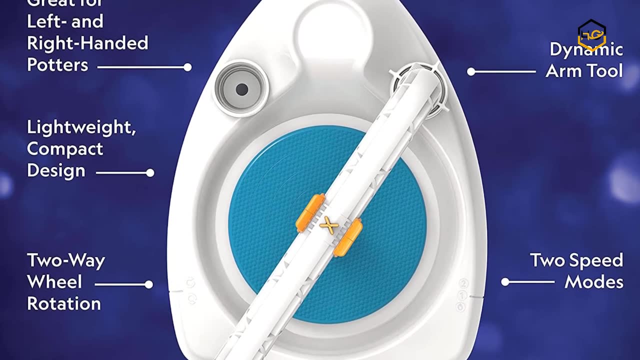 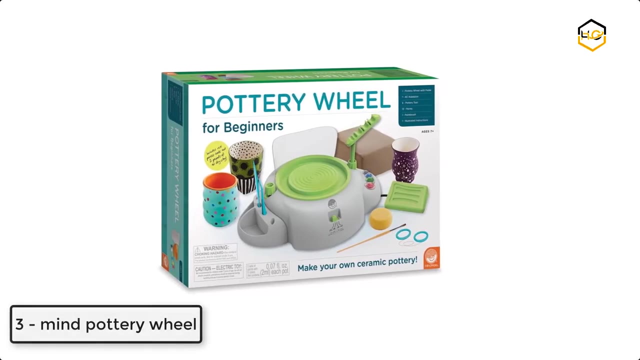 provides steady power and rotation against downward pressure with 2 speeds for different parts of the pottery making process. The detailed instructions include video lessons and helpful hints. to start, You can start kids off right, while the illustrated learning guide teaches the science and history of pottery. Number 3: we have Mind Pottery Wheel. The pottery wheel from Mindware is a wonderful way to 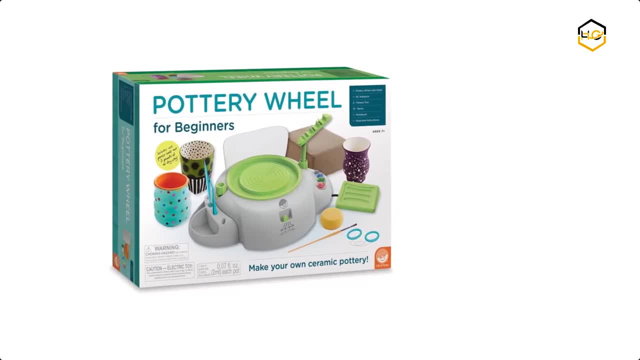 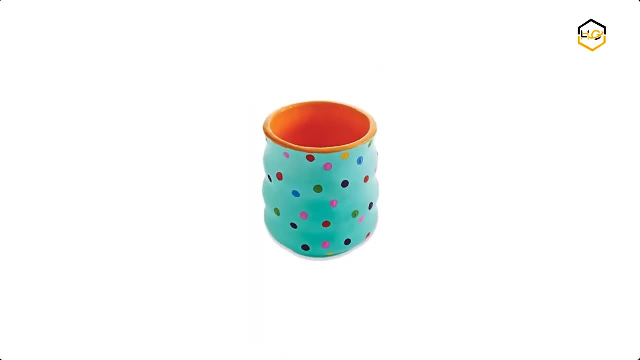 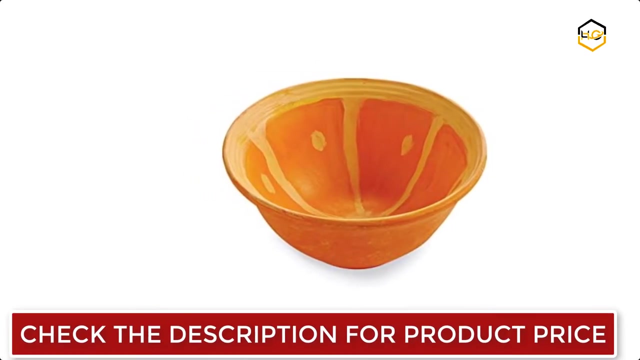 introduce children to incredibly fun and beneficial craft of ceramic making. This is the strongest and most durable pottery wheel available for children, making the process of creating fun throughout. It features a safety stop feature. prevents the motor from running if too much pressure is applied. that's helping you learn valuable pottery skills and preventing the motor from overheating.